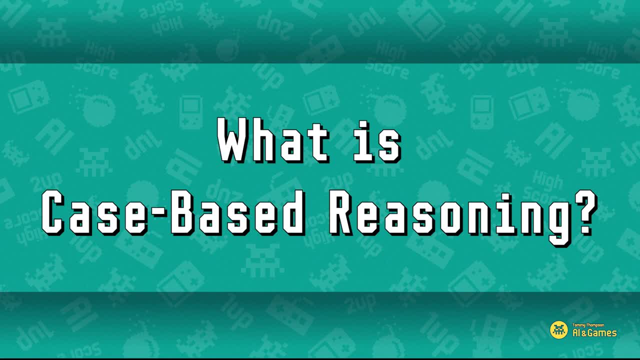 situation, we have one or more actions to resolve. The system is then focused on recognising the similarity of new problems to existing ones, but also how to manage that collection of accumulated data. While we are interested in the AI methodology, case-based reasoning stems largely from the 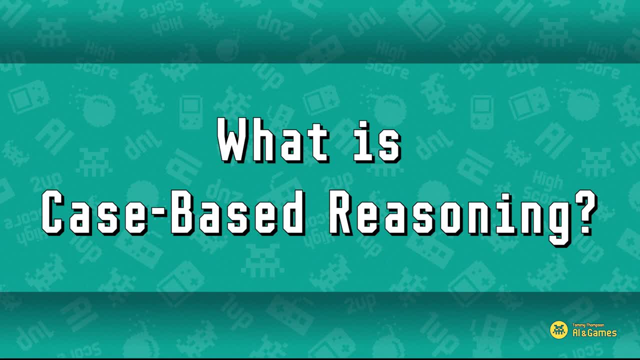 manner in which humans conduct problem-solving and has correlations within cognitive science. We face a variety of decision-making problems in every day of our lives, but seldom worry about how to resolve them unless they are entirely new to us, If we are, for example, 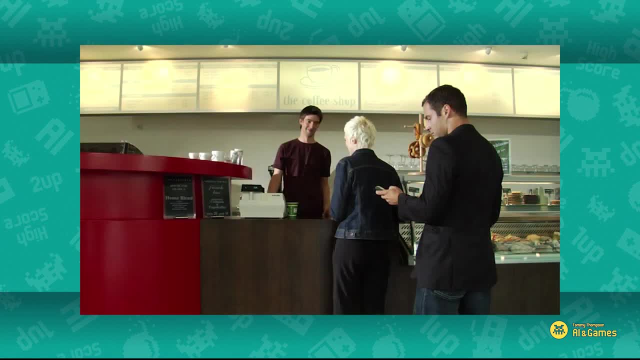 entering a coffee shop. We know how to get inside the building by opening the door. You don't question it, given you've learned at an early age how to open doors and, as such, getting into the shop doesn't prove a problem. You just open the door and go in and order your coffee. The door might 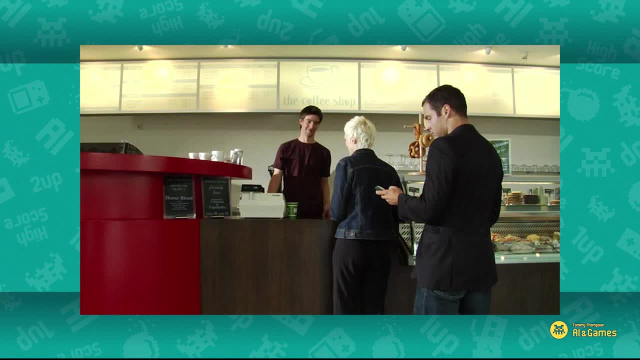 not look the same as other doors you've opened, but you understand that it's a door and know how a door works. Even if you're in a foreign country and don't know the language, you will approach the ordering of a coffee in much the same way you would do in your homeland. 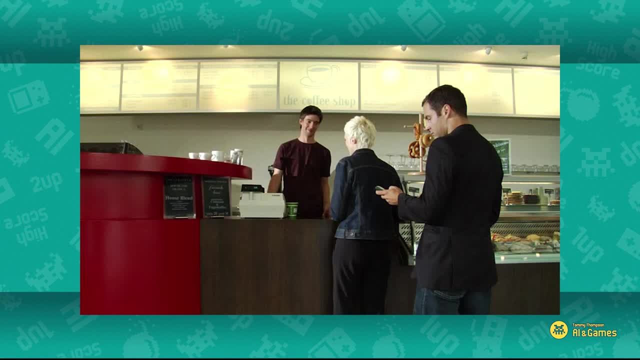 Given. the way in which a barista and customer interact during the transaction doesn't really change when ordering in a different country. The hard part is overcoming the language barrier at specific moments. In this case, you made a judgement based on prior knowledge to order your coffee in Paris, Rome or Berlin in much 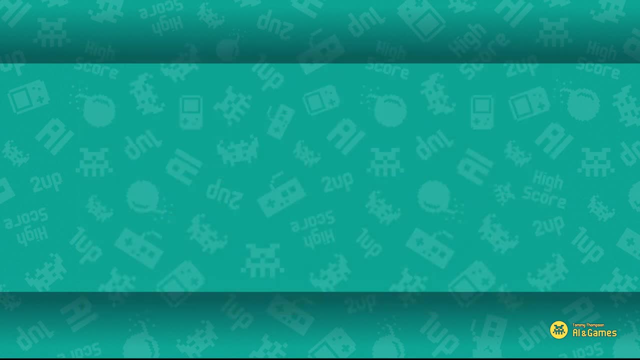 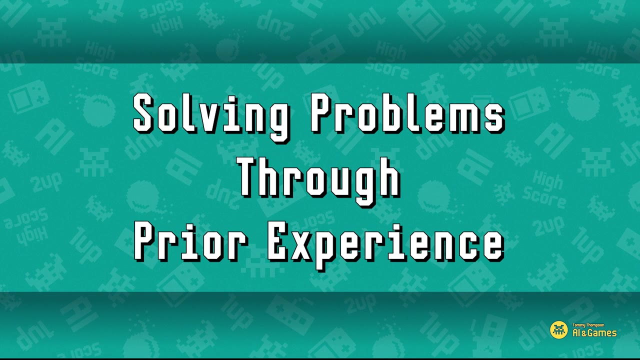 the same way you would do in your favourite coffee shop in London. I have solved this problem before, so I will do roughly the same thing as last time and try to work around the language barrier. The same principle often applies in video games with specific tropes. 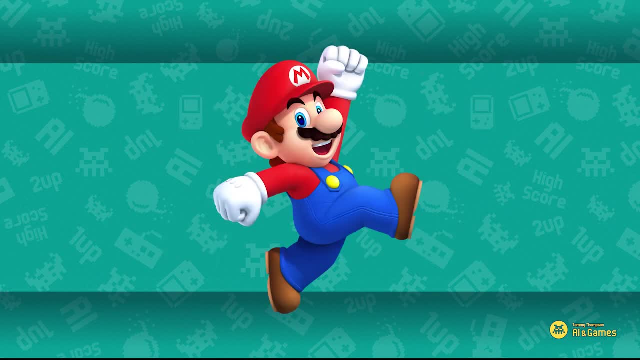 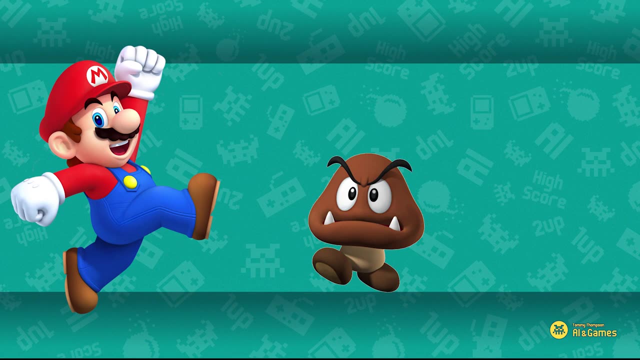 established throughout games, such that we repeat actions in the same or different game with an intended outcome. If we have an enemy moving towards us in a platforming game, we'll often jump over or onto it. We build an understanding of when jumping on an enemy proves to be the 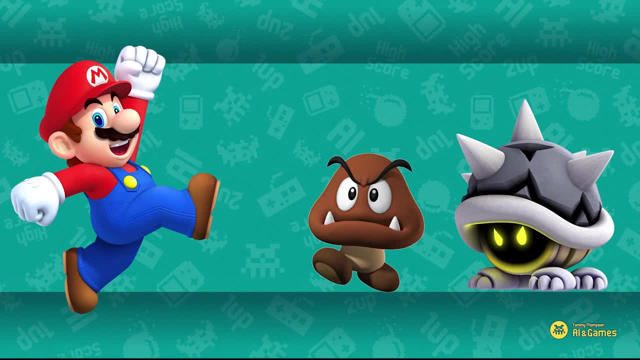 best outcome versus jumping over it. When we meet similar, albeit not identical, situations again in the future, we know how to tackle it. This is a critical aspect of how games are designed. We want players to memorise patterns of behaviour that yield positive. 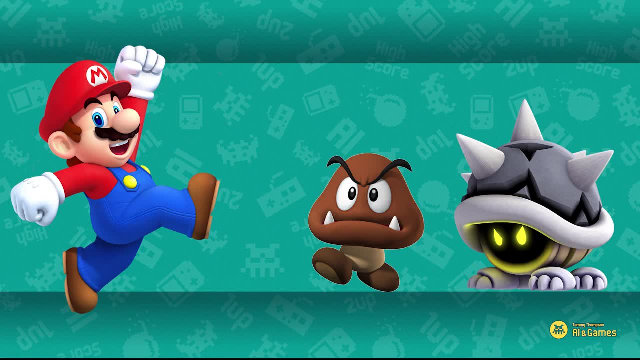 outcomes and make them repeat those patterns throughout the game in similar or different contexts. If this isn't properly established, the game can become confusing as we try to solve a puzzle that we're simply not prepared to deal with, as we've not had prior experience that 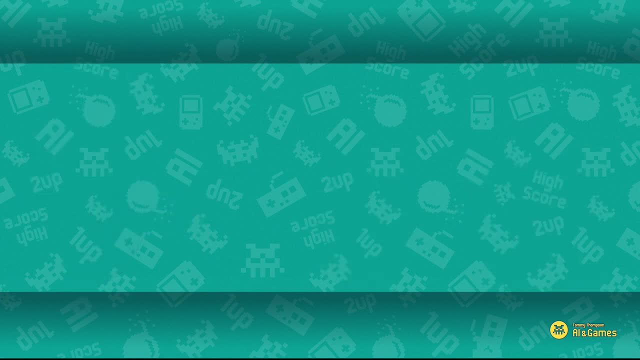 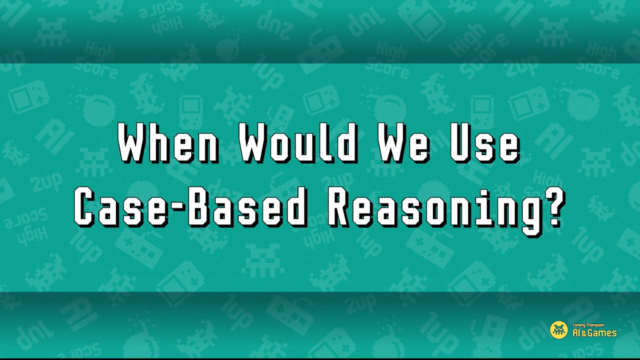 reinforces our understanding of the problem we're facing. Case-based reasoning is a good method to apply when you have a situation that requires diagnosis, prediction, classification or recommendation. As such, it is assumed a role in industries that has previously been covered by rule-based expert systems- a more rigid approach to the same problem that proved 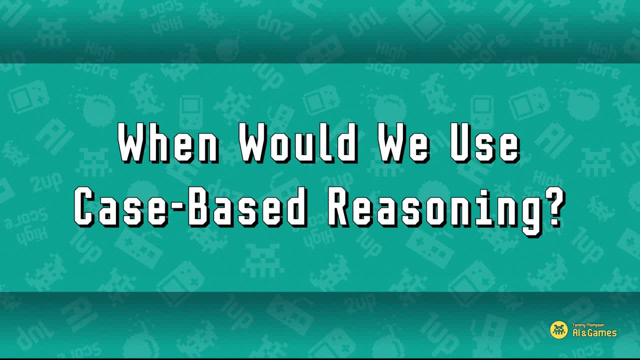 popular in the 1970s and 1990s. However, as we'll discuss later, CBR has effectively replaced them, given its ability to adapt and change its knowledge base over time. In addition, expert systems typically have a domain model where some high-level language is used to express data terminology. 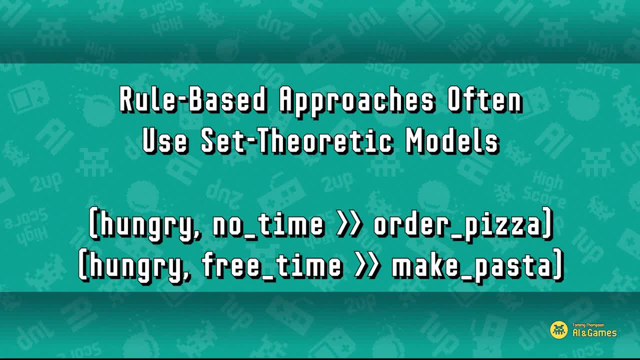 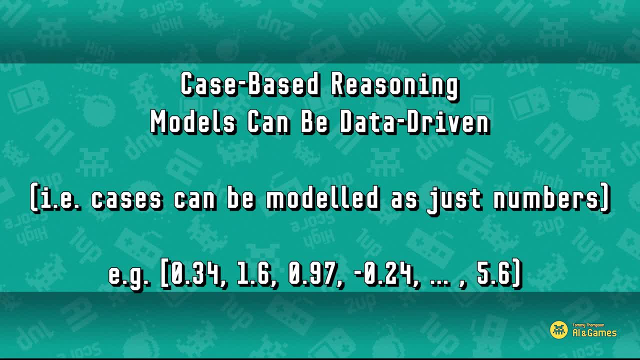 in a set theoretic language. Case-based reasoning doesn't require data to be modelled in such a way and can be far more coarse and data-driven, ultimately being reduced to a bunch of numbers. As such, there are applications of CBR in situations such as medical diagnosis vehicle. 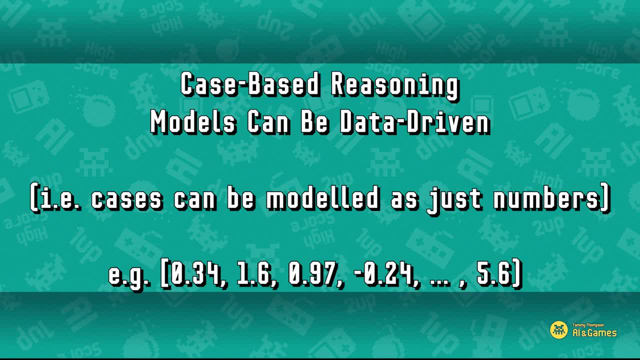 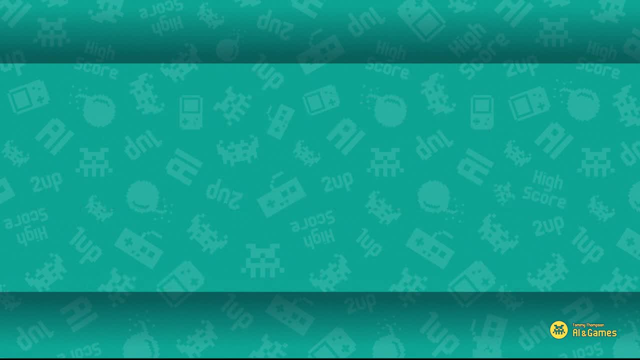 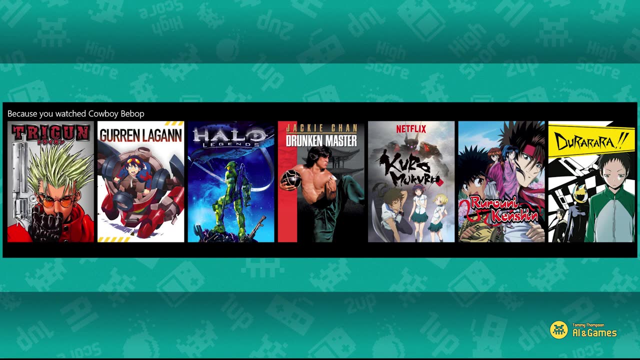 diagnosis and repair, anticipating court outcomes based on legal precedents and even fraud detection, given that in each case there is existing data that would allow us to identify what to do in a given situation or at least give us a rough approximation of how to approach a different, albeit similar, problem. Though perhaps the most common applications that 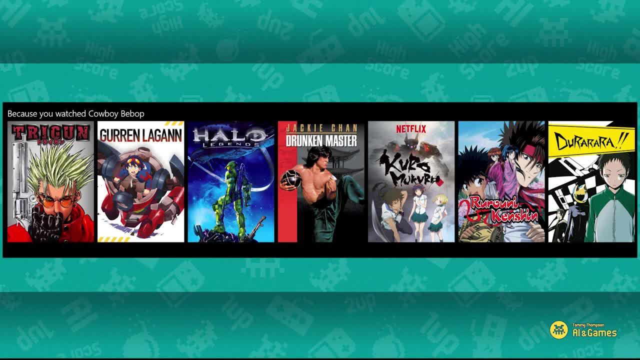 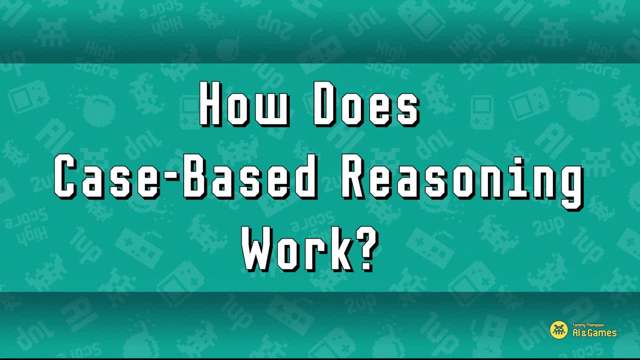 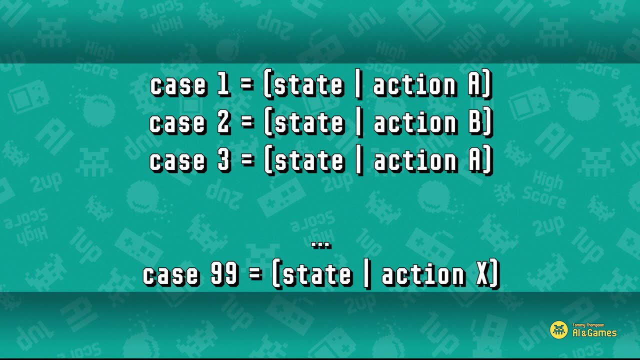 people are familiar with is the recommendation systems that you see in the likes of Amazon and Netflix. In practice, CBR is focused on the management of cases, a set of pairings of a given situation or state. So for this to work, case-based reasoning is structured as a four-step process. sometimes, 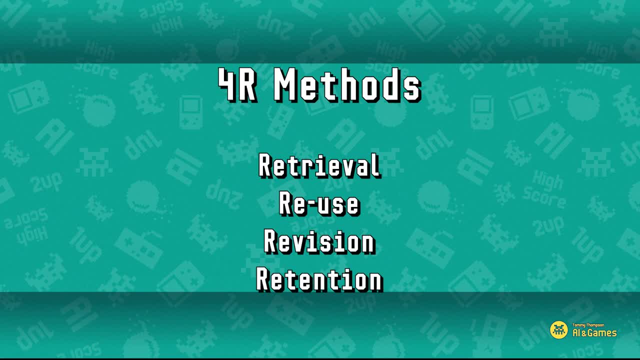 referred to as the four R's: Retrieval, use, revision and retention. Each of these phases interacts with the collection of cases, either editing the collection or retrieving actions from it to make. This means that the case collection is constantly being edited as the system is being searched for appropriate actions based 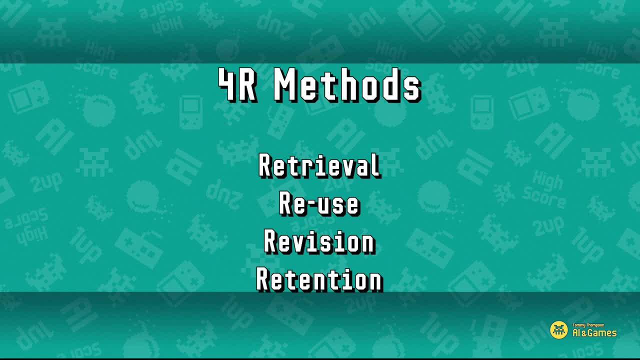 on current situations, combined with updating it to highlight whether a particular case proved useful in a given context, as well as adding new cases when it seems clear that the current situation has little relation to anything we've already stored. So to cover the four R's in a little more detail, 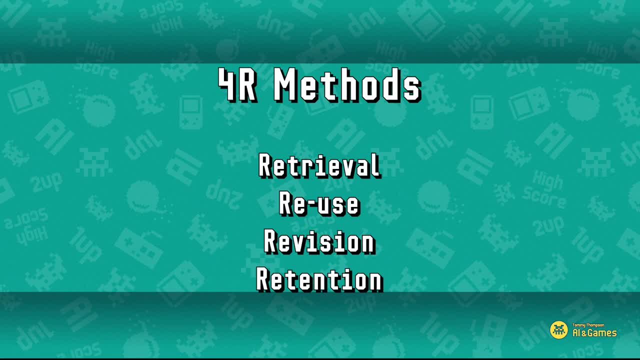 let's walk through each of them. Retrieval is the process of finding a case that is similar to our current situation or state. This relies on an ability to assess a given state on its applicability to the current one. We'll come back to this in a minute. 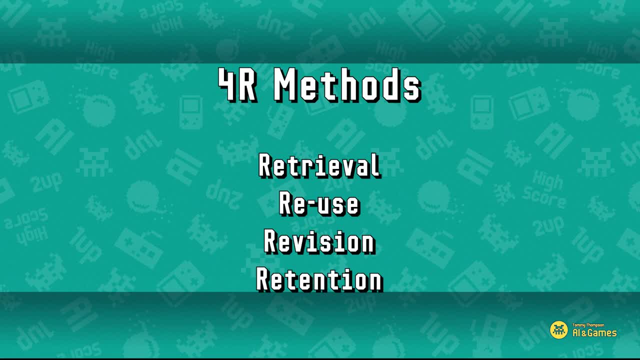 Reuse is when we retrieve a case and propose it as a valid action to apply in our current state. Revision is when we evaluate, through a series of metrics or even simulations, how well this proposed action will perform and whether it's practical to apply it in the potential future. 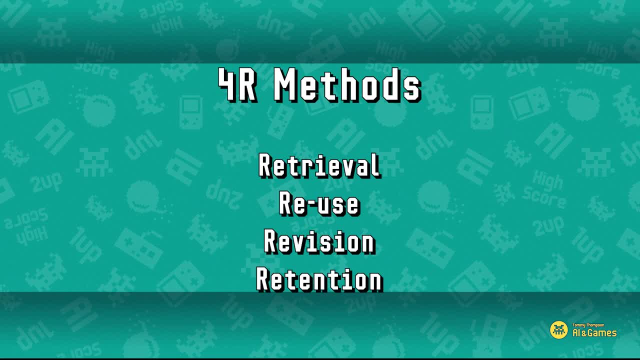 particular case we are in. This sometimes results in some revision of the action to fit the current context. Then, lastly, retention is applied after a successful execution, by storing the result of this experience in the case system. This is useful when we revise the proposed solution. 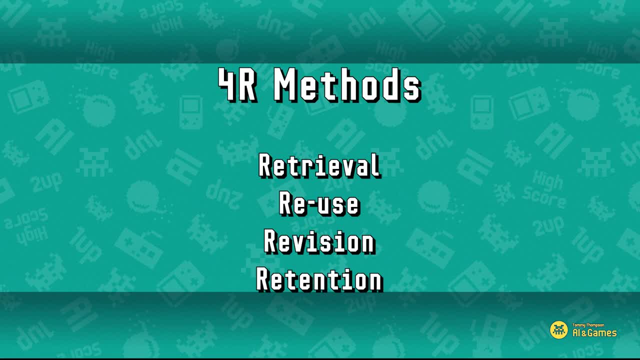 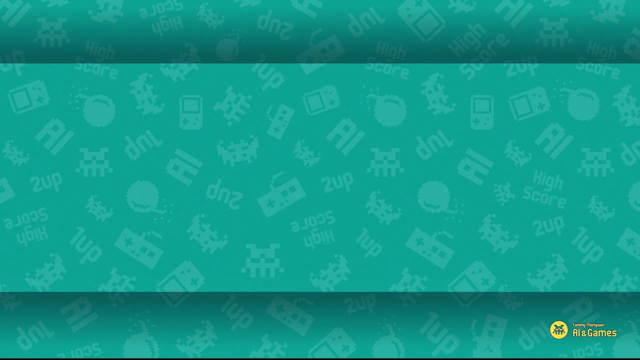 given it is now clearly an individual case. These 4R methods provide a decision making system that can generalise its previous experiences, allowing you to apply decisions made in similar but not identical circumstances to new situations. Coming back to the coffee shop example, you can continue to open that door and order your 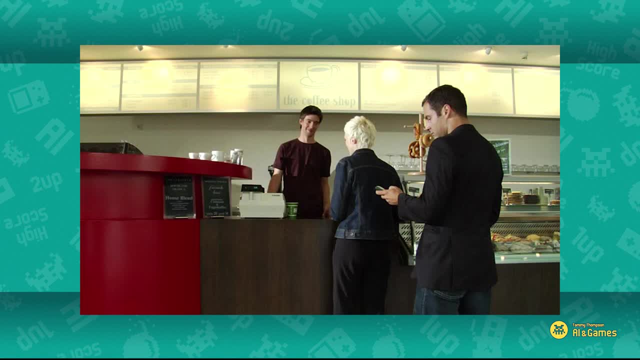 coffee, irrespective of where the door is in the layout of the coffee shop, because it's roughly the same problem each time. We've successfully generalised this problem. Even when the situation differs, like you're baking different types of cake, you can often apply. 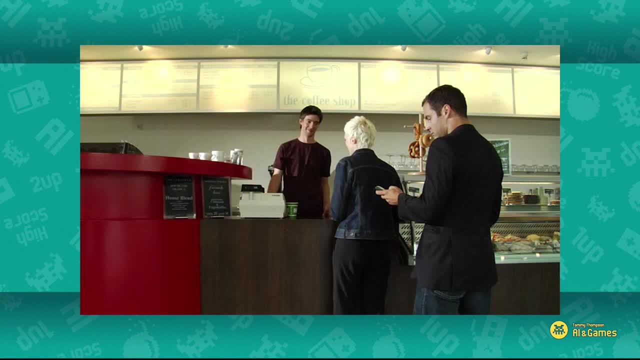 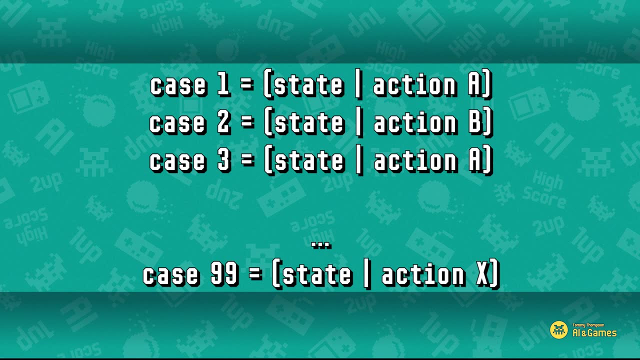 the same rules to get your desired outcome given. once again, you've generalised that problem. The secret sauce is how the model is stored and your metrics for comparing cases in the system, as well as comparing cases to the current state of your problem. We would typically store the 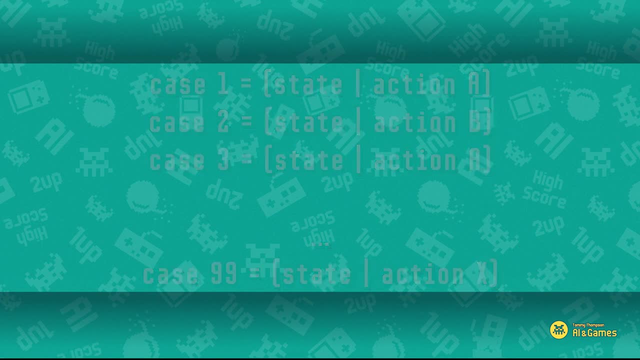 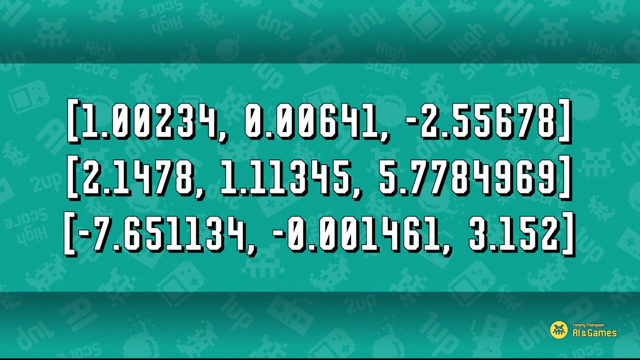 states of our case bases as n-dimensional real vectors, or rather one or more collections of real numbers. This is useful, given it allows you to quickly run similarity measures across two distinct cases to check whether they're compatible with one another. These similarity measures often act like heuristics in classic AI search, given that the case is not a single.